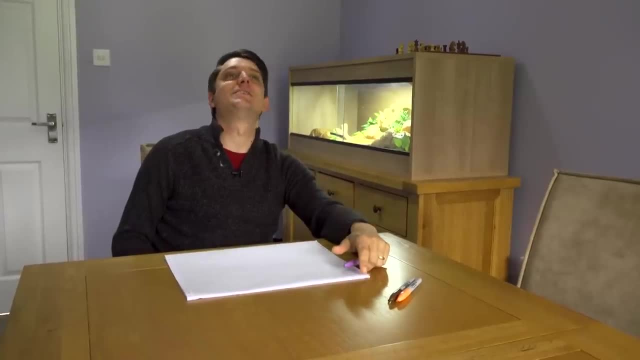 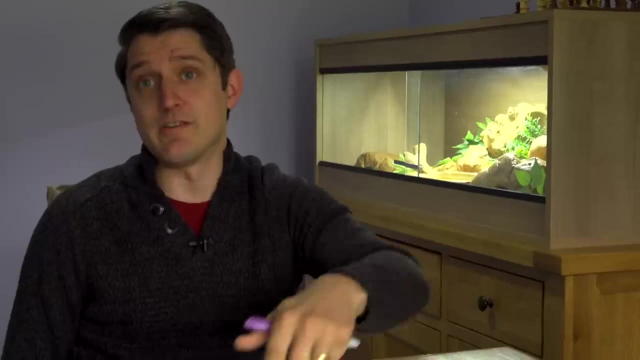 just turned a computer on after a week or something like that, and and so it doesn't know where google dot-com is. It will have to make him a DNS query to find out what it is. Now the first point of contact will usually be a: name server that belongs either to you know your organization that you're in. so let's say the University of Nottingham will have a name server or two, or it will be your ISP, if you live at home, probably, or you might have configured something like open DNS yourself and you might have one yourself. But let's assume. 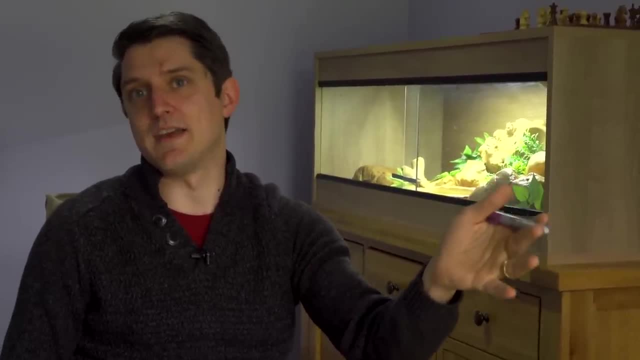 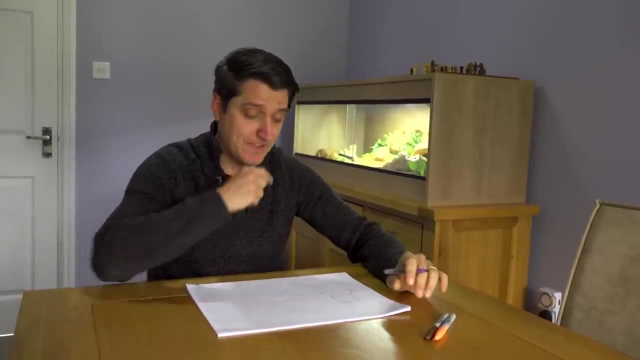 before for the sake of argument that we're using- I don't know- our ISP's domain name server. so so this is our computer here and we want to go to some website, so let's say googlecom. now we don't know what the ip address is of googlecom, so we're going to have to ask some. 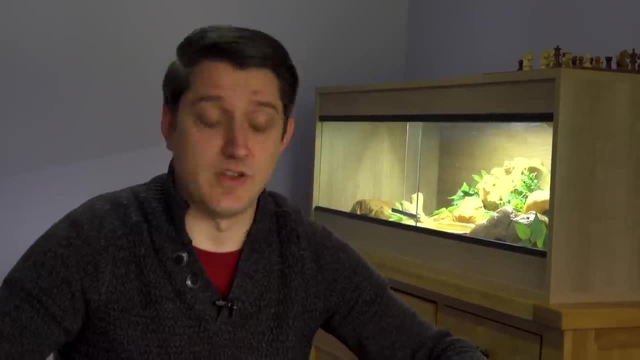 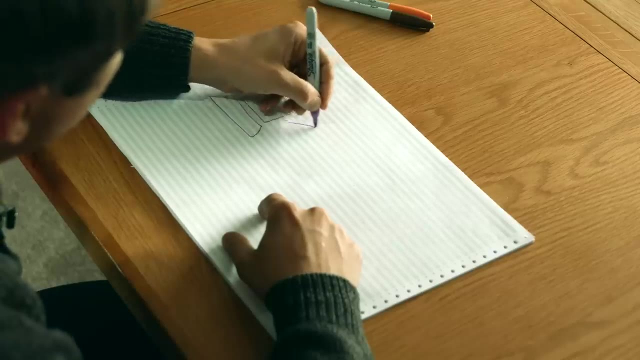 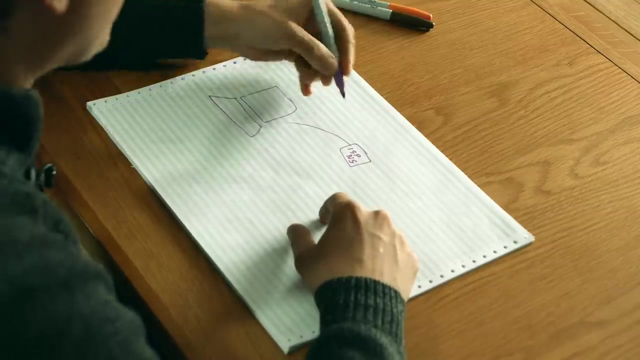 other computer that might know. what would normally happen here is. we would ask a name server that we've either configured ourselves or that is, let's say, given to us by our isp right. so i'm going to connect to my isp server here- isp and this is their name server- and i'm going to say googlecom. 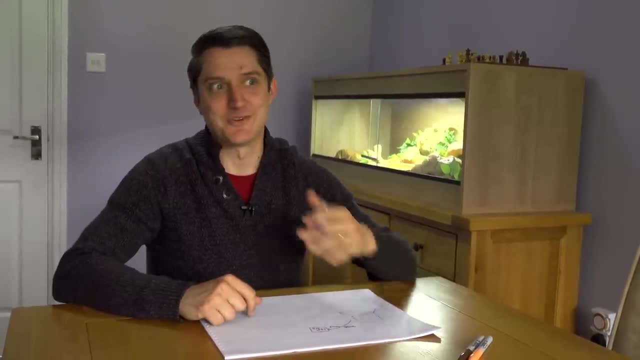 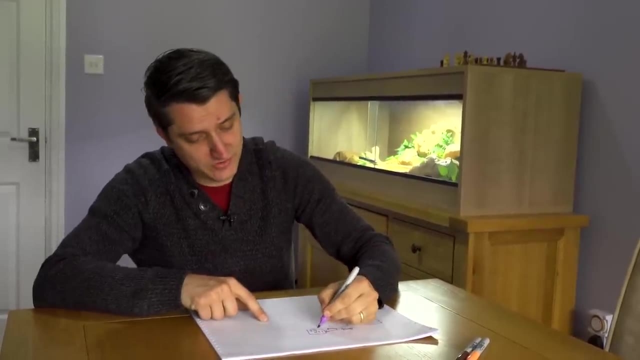 question mark right? i mean there'll be a few other bits of information in that, not just googlecom in its rhetorical question. um, now, this server will either know- because it has a little cache of of stuff that it can look up right now- if someone else has been to googlecom recently. 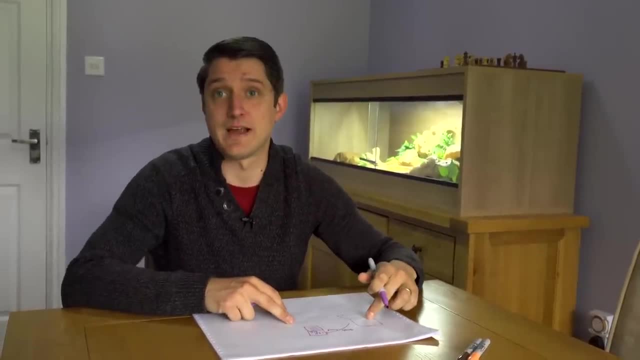 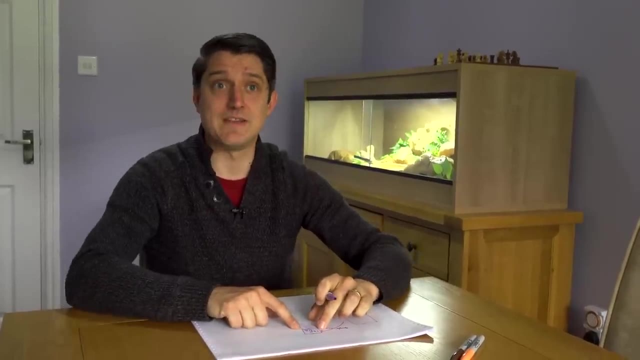 which is obviously quite likely. it would know what that is and it will give that information back. but let's assume that it doesn't, um, and let's also assume that this is set up to be what we would call a recursive resolver. so that means it can not only answer queries about dns, but it can also ask queries about dns. it's. 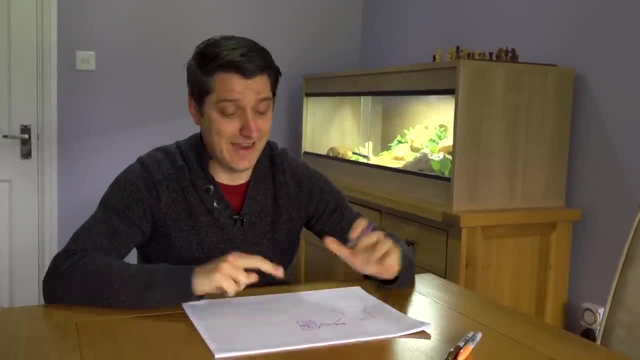 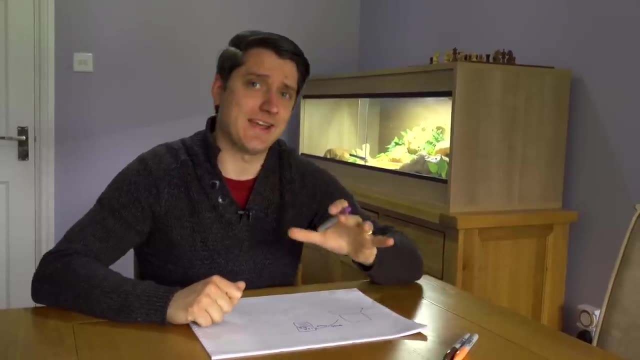 got to ask another machine that it thinks might know the answer. now it hasn't got the foggiest idea right, because there are a lot of different ip addresses. so what it's going to do is it's going to pick from a list of root name servers, right? so it's going to talk up here. on the internet to a root name server, so the name server will go off to the root name server of, which is about 20.. now these are hard coded, right. all computers have access to these, um. i think one of them is run by verisign, for example. one of them is run by nasa, right i? i don't know why, um, but it is. so, um, this root name server will say: i don't know, right, i don't know what googlecom's ip address is, this this day, right, because they maybe they turn their computer off and on again and it's changed. but i do know, is that this ip address of this global top level domain name server could help you? 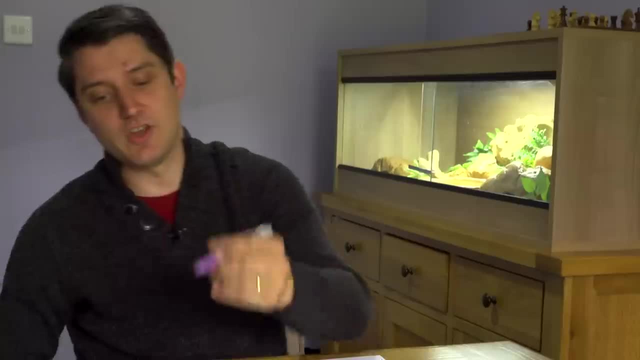 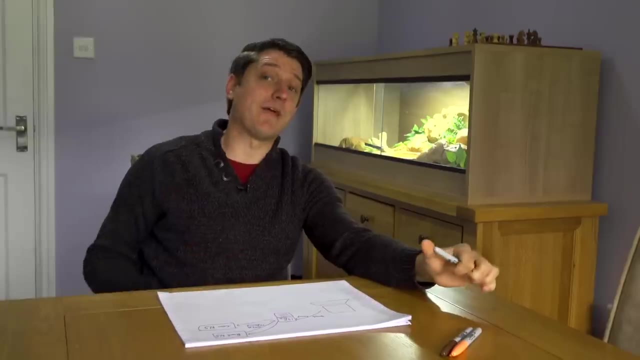 right, and there might be a few of these as well. so it's going to send us a dot com name server right, or multiple ones, and one will pick one. now, this dot com name server- we're getting a little bit closer, so it's kind of working our way backwards through the url in some sense, or through. 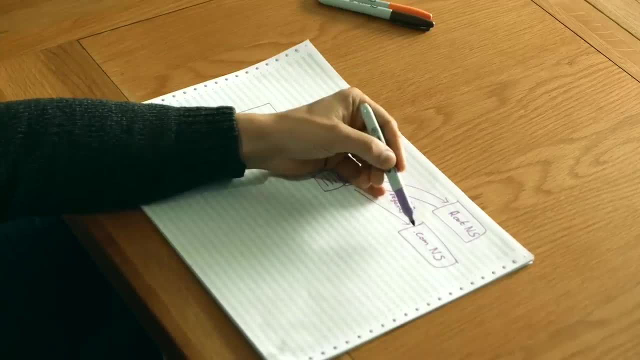 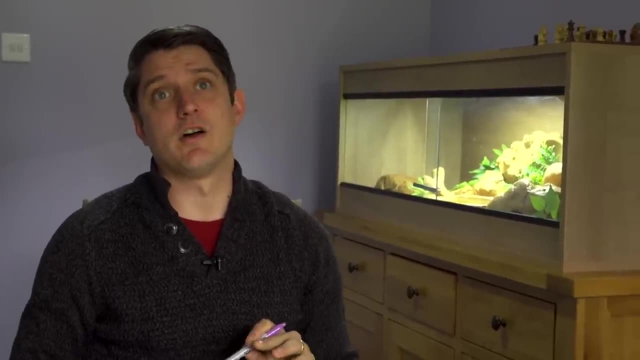 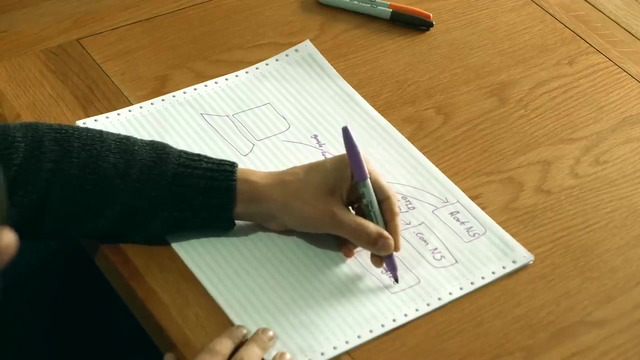 the domain name. so we will put in a request to thiscom name server. it will say: i don't actually know that. the next place you should ask, or the kind of the name server that's responsible for this zone, is, let's say, ns1.googlecom or something like that. now we're getting a lot closer right. 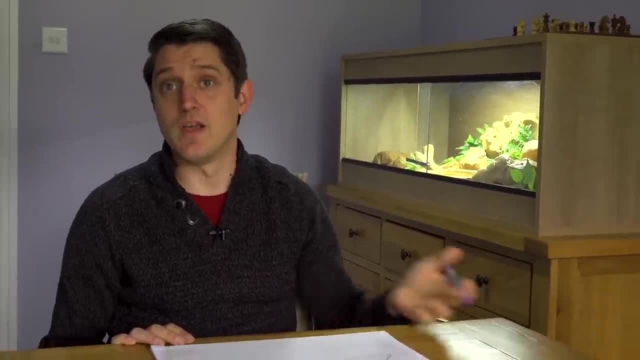 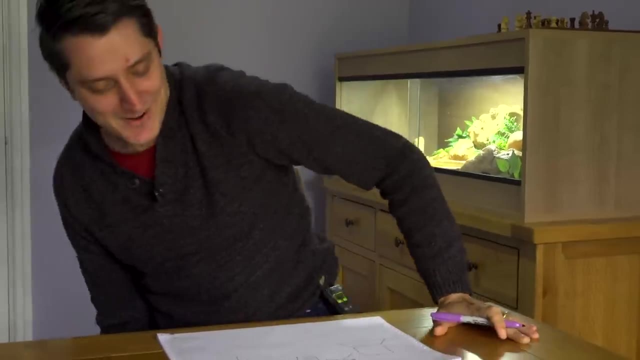 this is a good a name server, let's let's say hypothetically, it's run by google. they're going to know what their own ips are, right? if they don't, then google isn't going to work right. this is like lesson one of web web administration. so we actually put in a request to ns1.googlecom this. 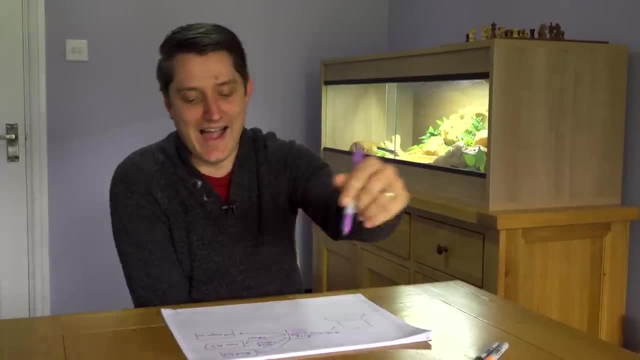 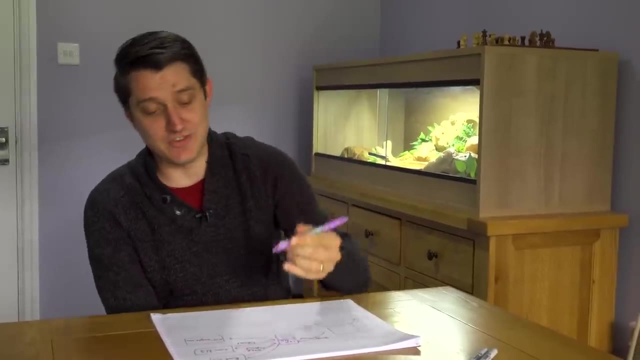 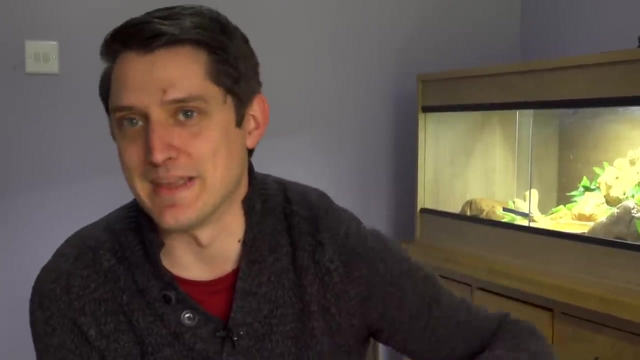 is what we're going to send back to google, sort of spelt right with a bit of a mess with my pen, and they're going to send back. when we actually query ns1.googlecom- what is googlecom, it will finally actually tell us it is, you know, 10.0.1.2. right now it definitely isn't that, but you know. 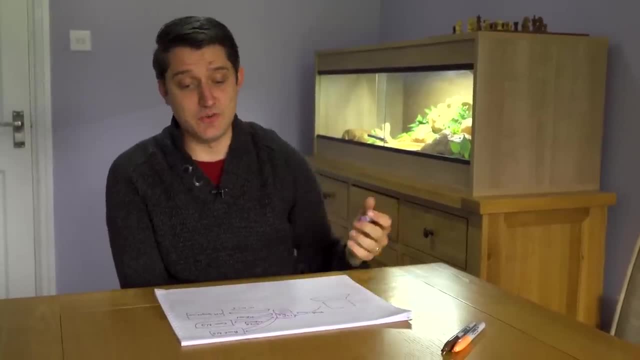 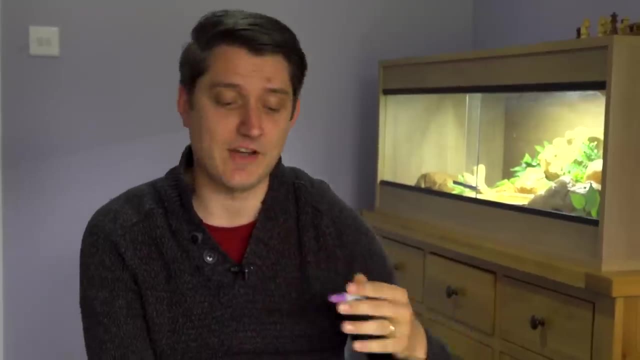 it, could you know? that's the idea. so we finally have an ip address now. what we can actually do now is send an http get request or a ping or whatever it is we want to do to that ip, and then that's how it works. now the dns service is a little bit more clever than than this sort of. 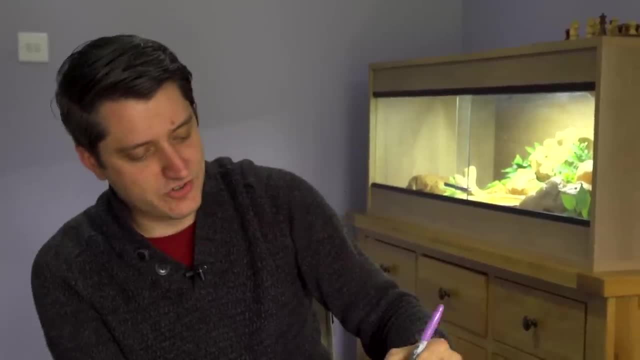 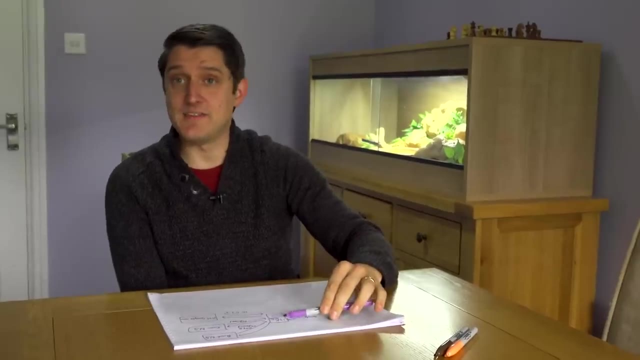 overview right, because of this caching and stuff like this. so i have a cache here and this recursive resolver will also have a cache and any other resolvers involved will also have a cache. let's suppose that this isp's name server is serving 10 000 customers, right, all of whom are? 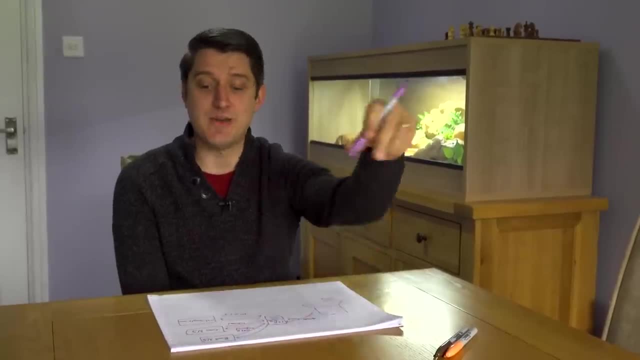 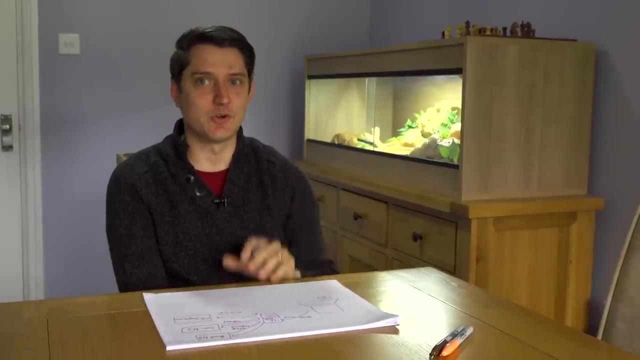 going to google. this is a bit of a waste of time, right? especially given that google probably not changing their ip every hour, right? so the first person in the morning that gets up and goes to the googlecom is going to have to wait fractions of a second longer, right, because it's going to be. 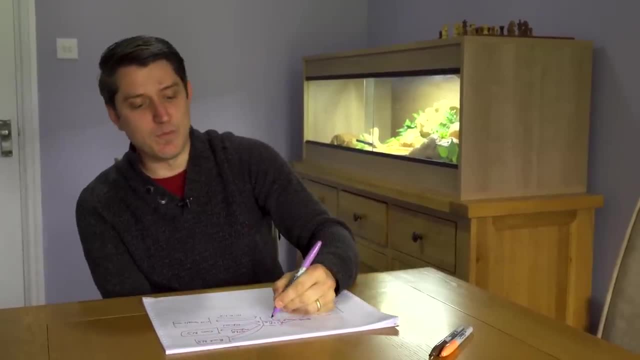 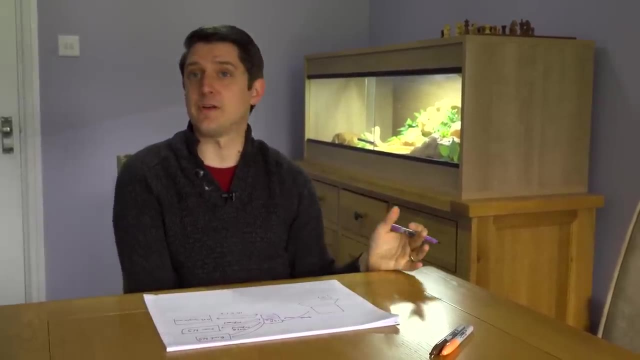 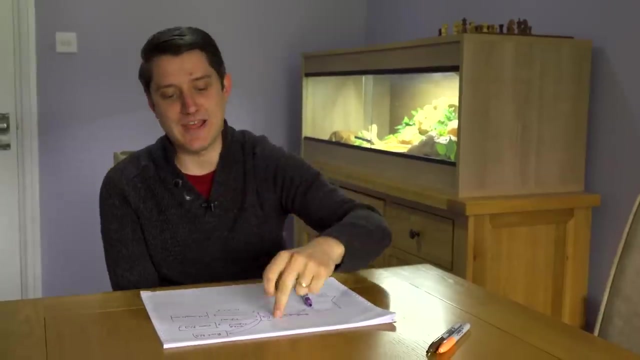 doing this, um, but then googlecom will be put into this cache with a time to load, time to live, and then for that amount of time. this will just serve that straight back, right? so what is googlecom? it's this, right. it's 10.0.1.2, whatever, and that means that this, this name. 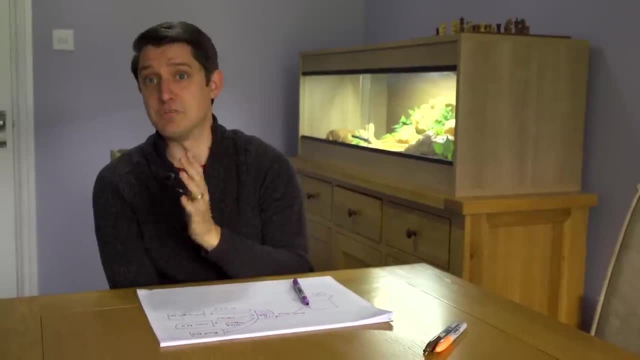 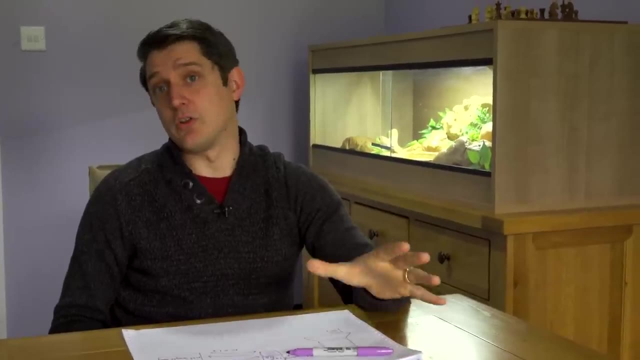 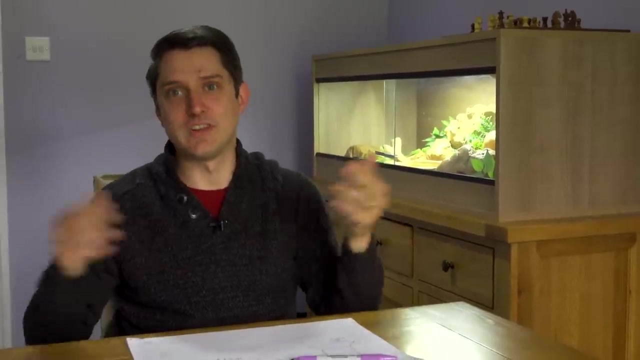 server, which will be quite powerful, can serve all the isp's customers really really quickly, right, which is kind of neat. this is basically a distributed database. this name server is going to be putting in lots and lots of requests right to hundreds of servers, probably per second, because of all the people on the internet asking i want to go to random. 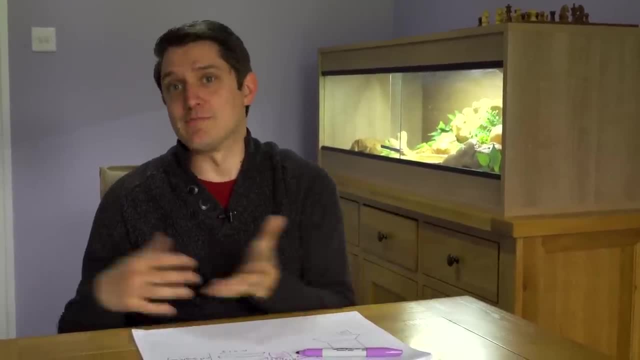 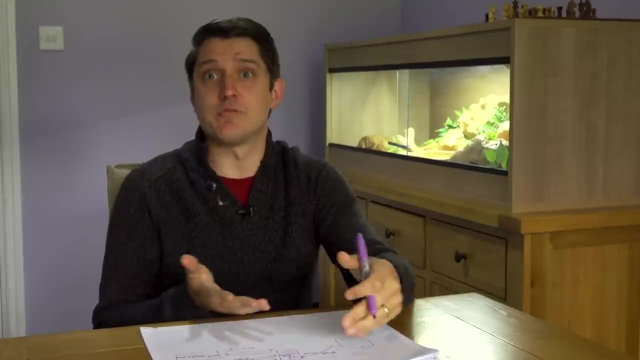 websitecom, randomwebsitecom, websiterandom and so on, and it's going to be doing all this. how does it know what to do with any of this? all this gibberish of information is coming back. well, what it does is it has a query id which it sends out whenever it sends out a request. 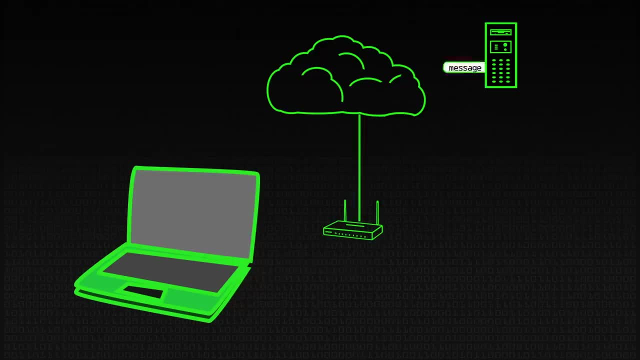 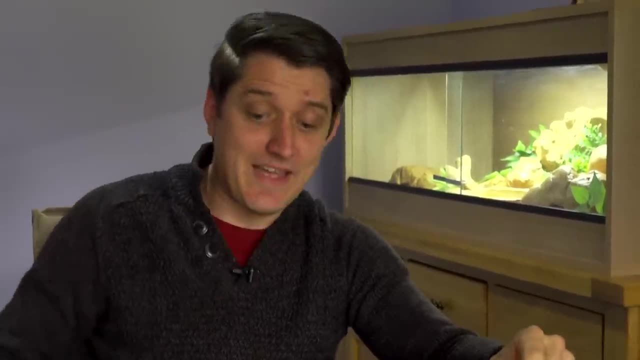 and the name server that responds will respond with the same query id. so it's labeled, it's labeled right, so, and that allows it to sort through the mess a little bit more. um, it leads to a slightly interesting quirk, which is that if i send a, 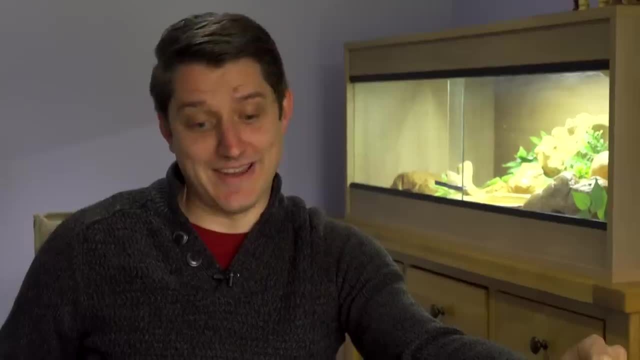 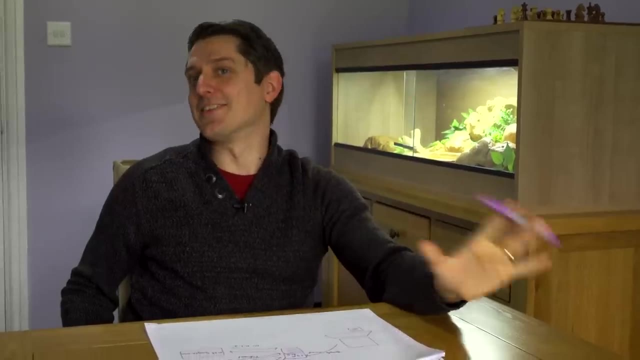 response to a name server but it didn't want. but i get the query id right, it will accept it right, which is for a different video. that's dns cache poisoning. for the most part that doesn't happen right. for the most part the query id is matching. if it works out quite well and it's really really. 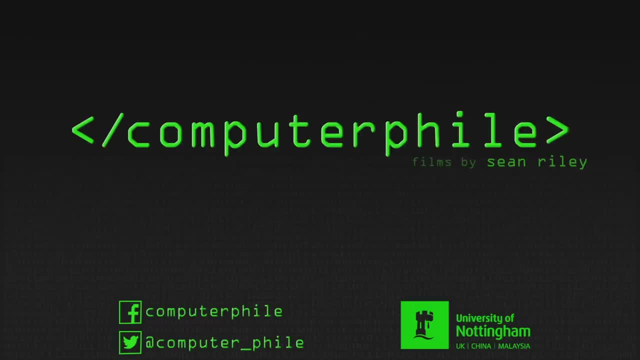 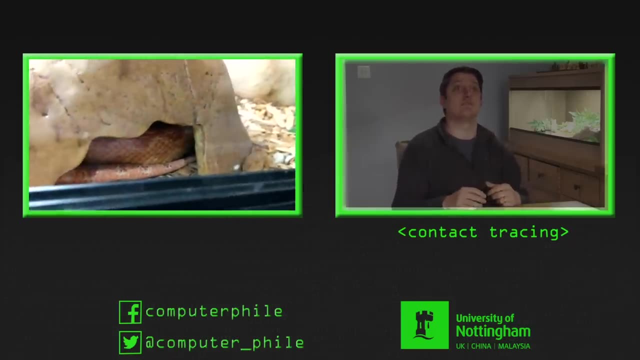 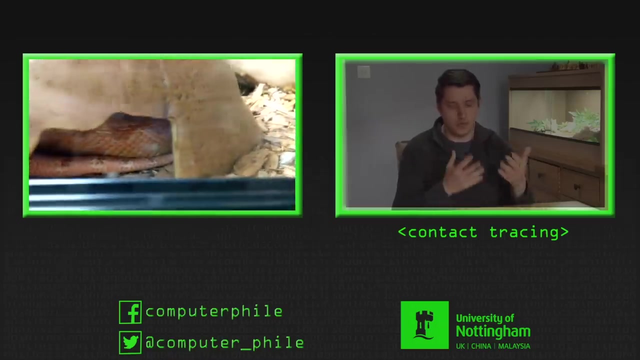 quick. so what is she? she's a corn snake. i'll be no corn snake, but she's in the middle of shedding and she's. she's grumpy and hiding under a rock and probably asleep. so you know, that's, that's the best of you you're going to get at the moment. we might see her another time. yeah, that's right.